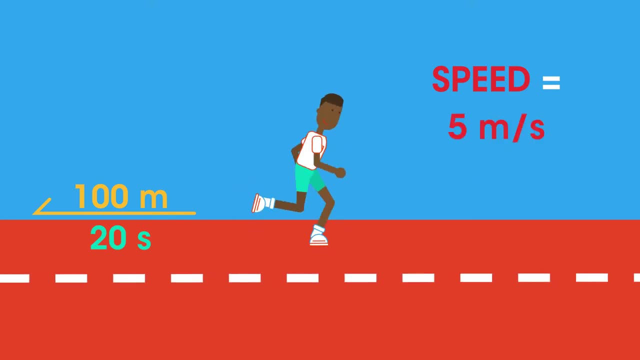 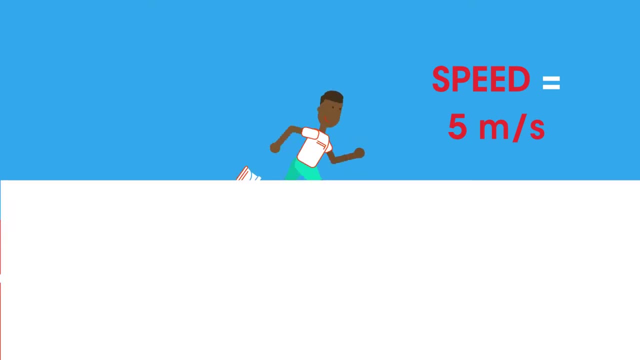 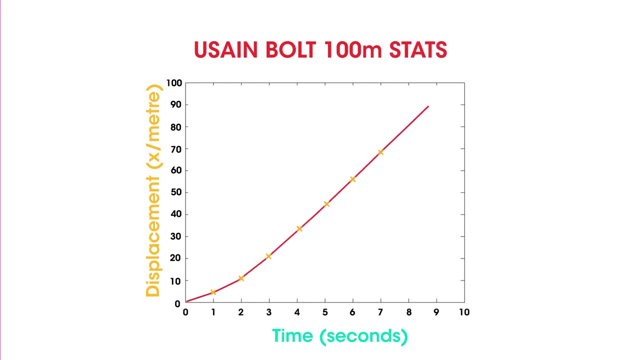 by 20, or 5 meters per second. However, this assumes that the man is running at a constant speed for the entire race, But this is never the case. Look at this graph of Hussein Bolt. Notice it takes time before he reaches his maximum speed. In a longer race, you might start off very 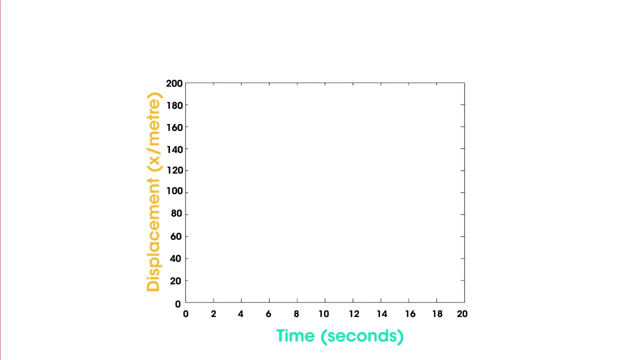 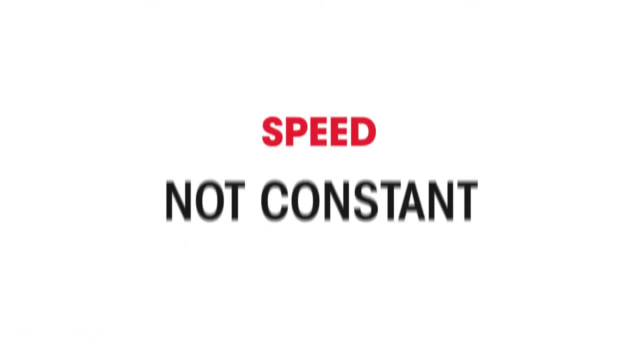 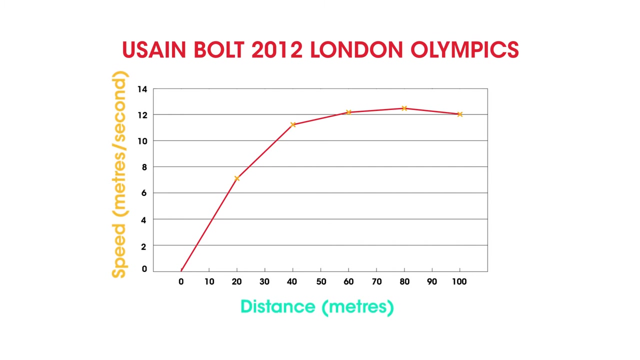 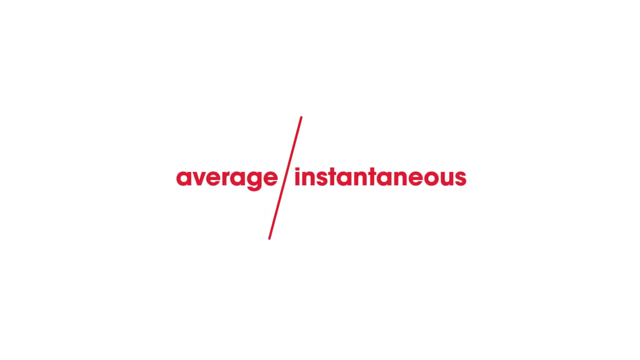 quickly, but end up slowing down as you get tired, And in some races, runners will speed up right at the end. All of this means that our speed is not constant for the entire race. This is Hussein Bolt again. This is where we need to consider the difference between average speed and instantaneous. 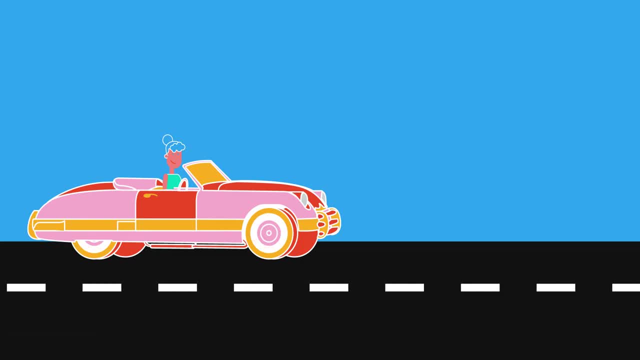 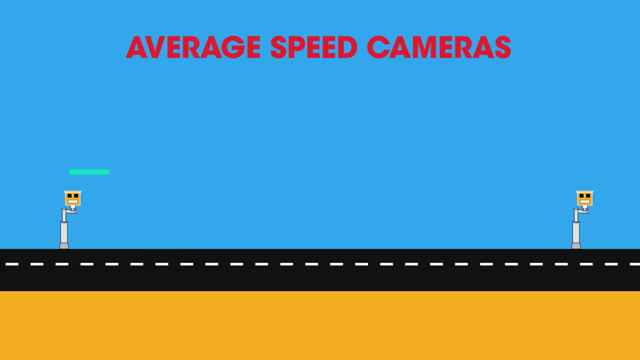 speed. Consider a car. A speed camera detects its actual speed at the time it passes the camera. It's instantaneous speed. However, there are now average speed cameras operating which record your time to travel over a long distance. Cars are less likely to speed in this case, as to avoid being fined, they would 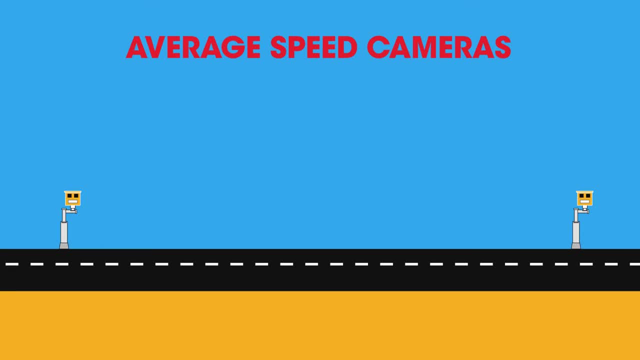 need to then drive more slowly to lower their average speed. But today we're only going to consider how to calculate the average speed. Let's look at an example. A dog is running across a field. She runs the first 50 meters. She runs the first 50 meters. She runs the first 50 meters. 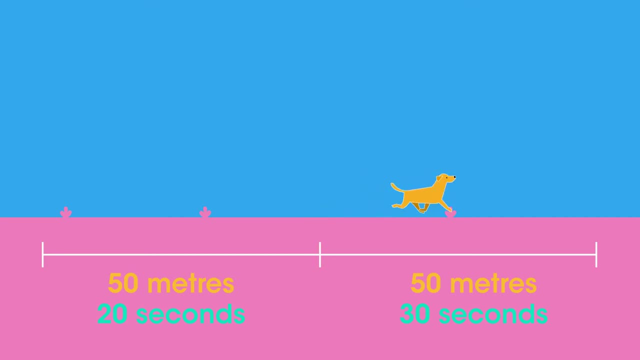 In 20 seconds, but then gets tired and runs the last 50 meters in 30 seconds. To calculate the average speed we must first find the total distance the dog has traveled, Then we find the total time the dog has traveled for. Then we can calculate the average speed by dividing the total. 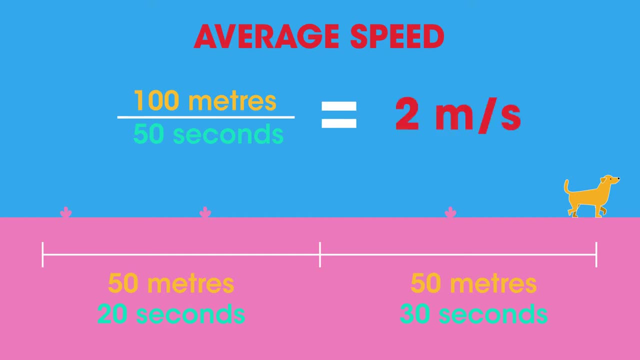 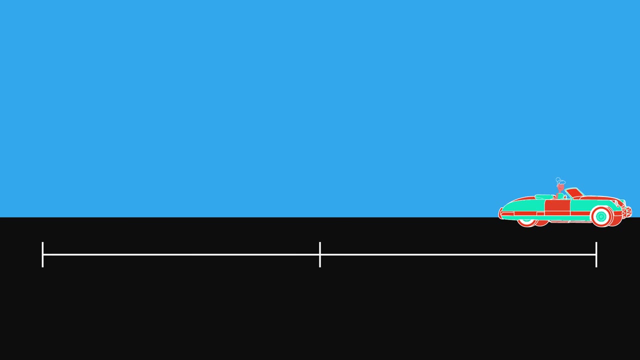 distance by the total time. Simple. And now it's your turn. Here's another example, This time a car traveling down the road. The car travels 450 meters for the first 20 seconds, but then it hits some traffic and has to slow down. It then travels just 150.